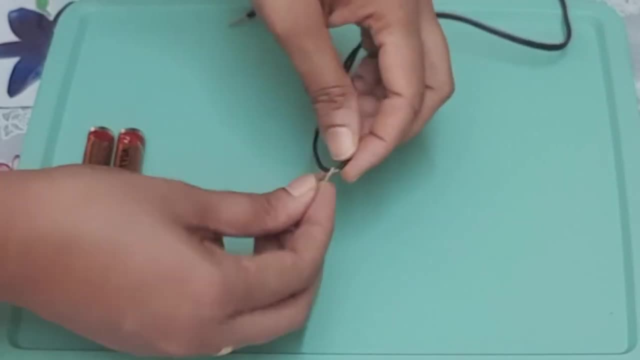 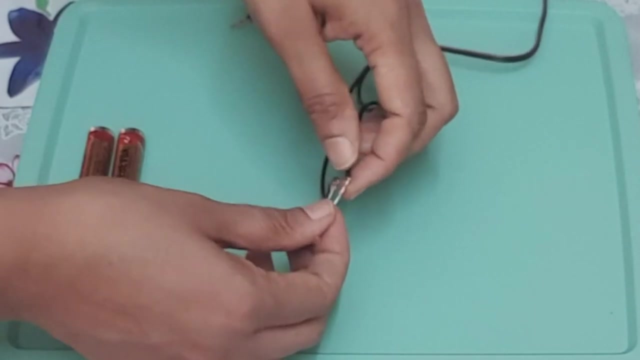 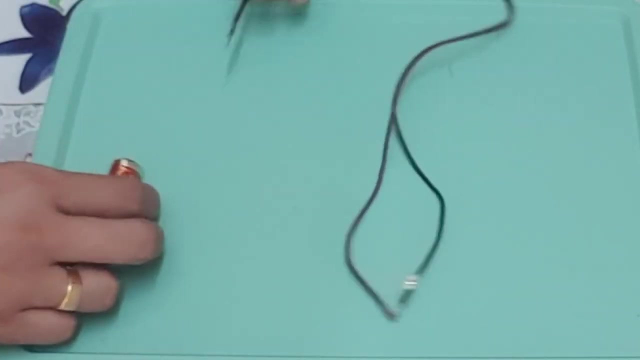 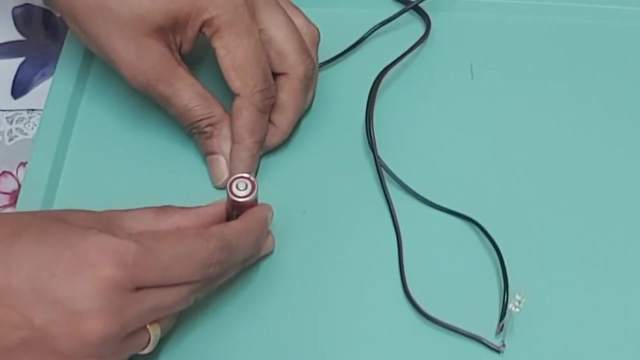 other two of the bulb. You connected one terminal of the electric cell to the other terminal through wires passing to and from the electric bulb. Two terminals of the electric cell are connected to two terminals of the bulb. Such an arrangement is an example of an electric circuit In an electric 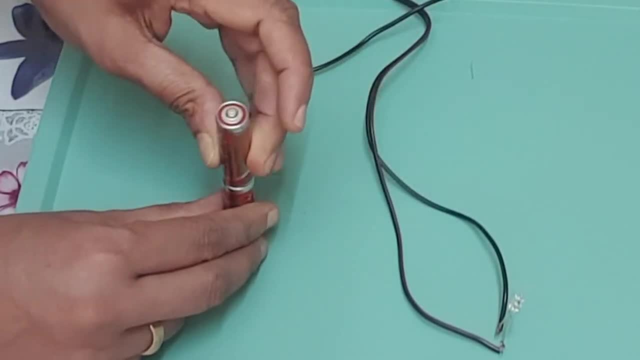 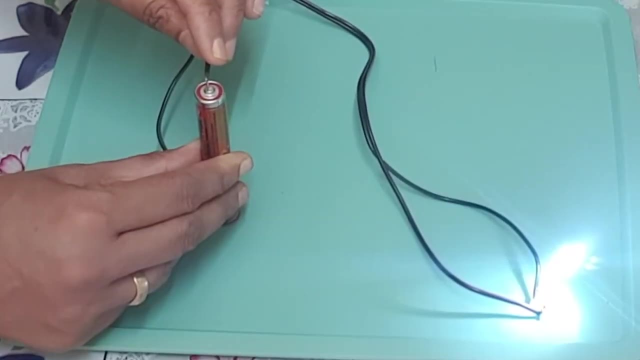 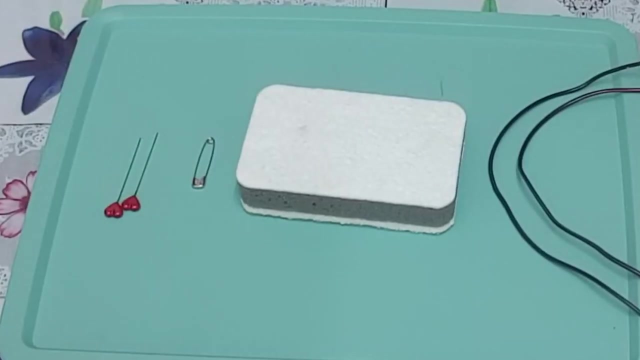 circuit the direction of current is taken to be from the positive to the negative terminal of the electric cell. Dear children, we can make simple and easier switch to use in our circuit. You can make a switch using two drawing pins, a safety pin, two wires and a small sheet of thermocol or a. 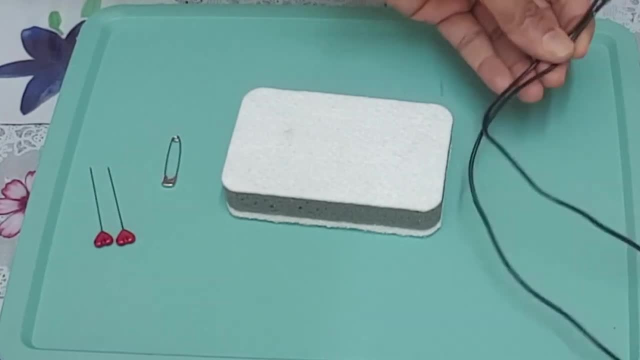 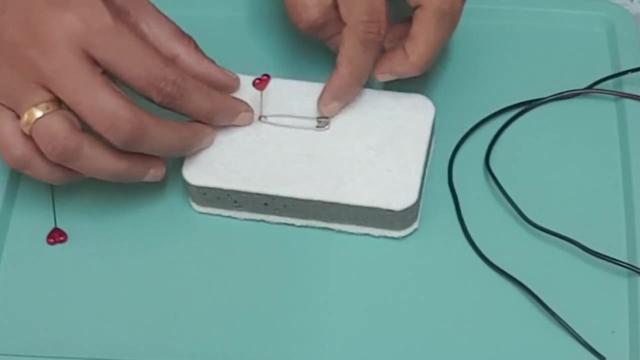 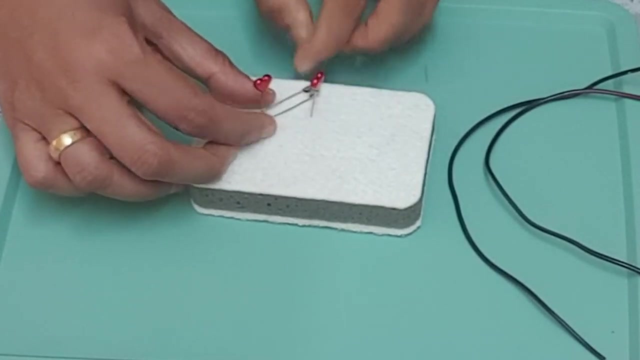 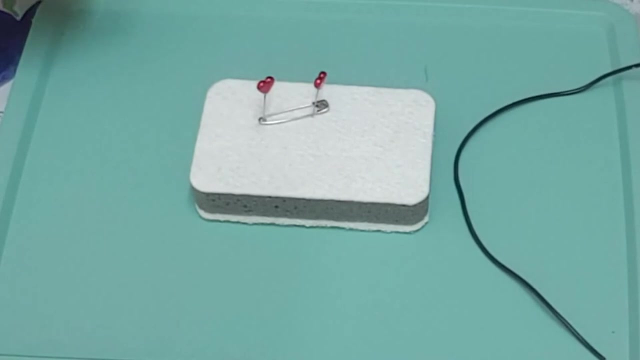 wooden board or sponge. Insert a drawing pin into the ring at one end of the safety pin and fix it on the thermocol sheet. Make sure that the safety pin can be rotated freely. Now fix the other drawing pin on the thermocol sheet in a way that the free end of the safety pin can touch it. 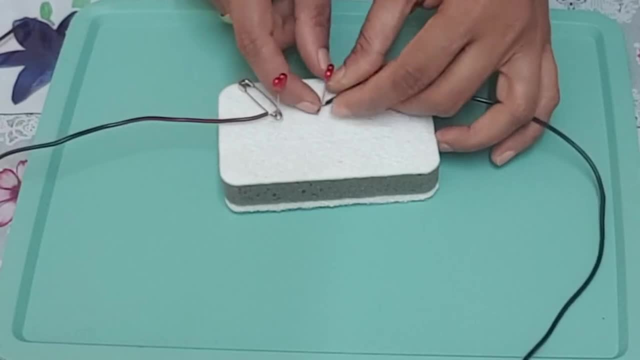 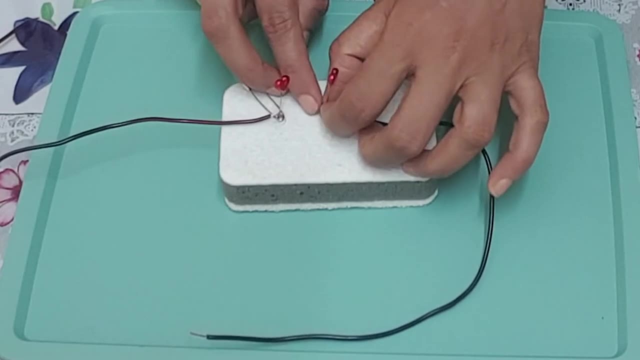 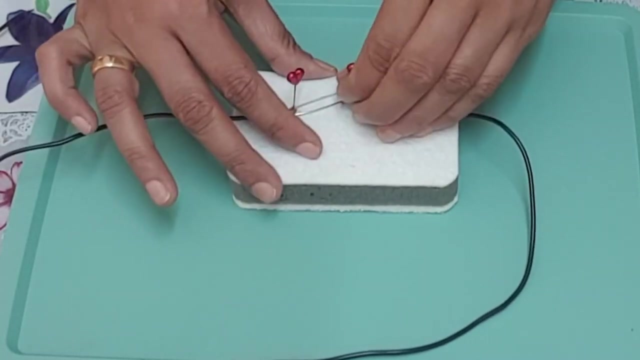 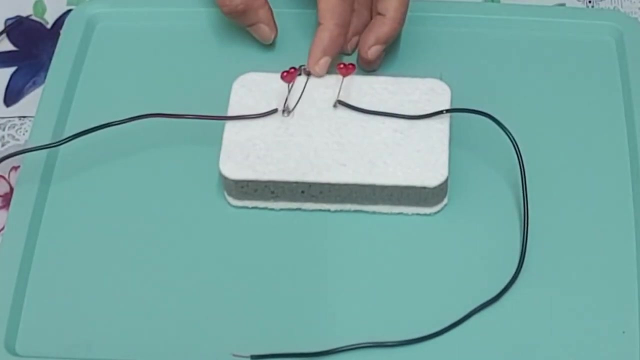 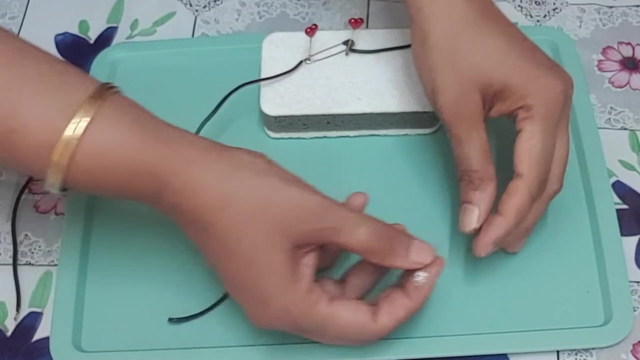 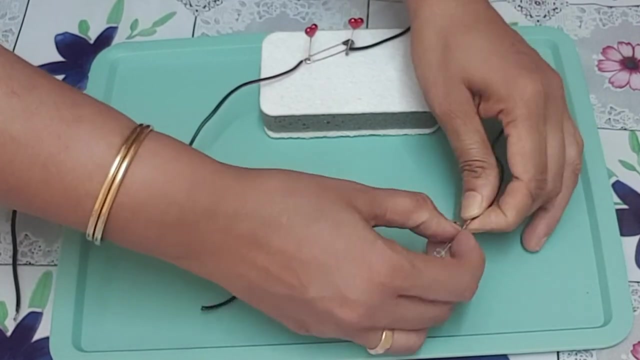 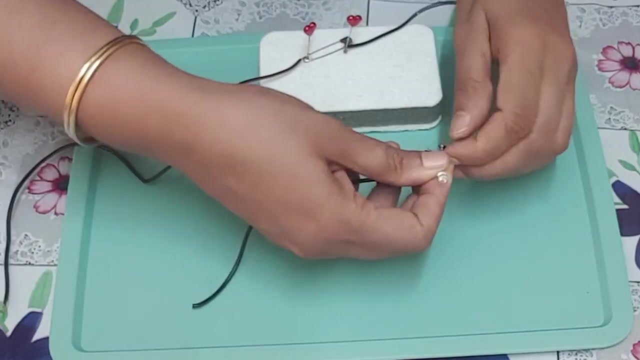 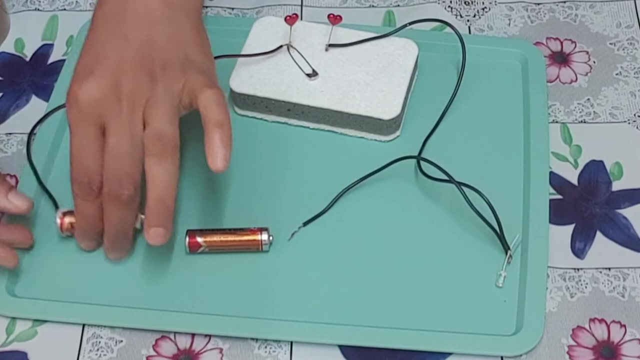 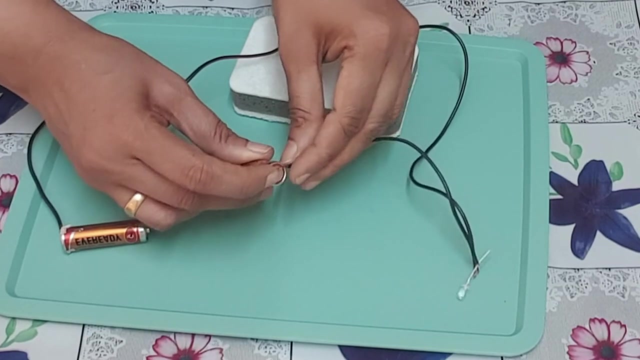 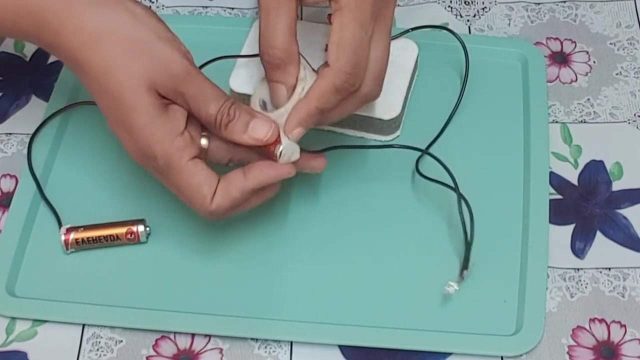 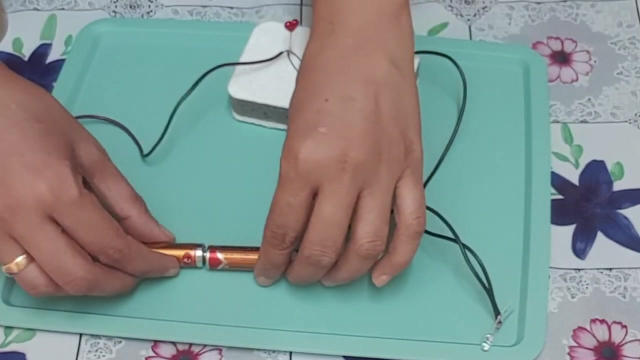 Now stitch the other drawing pin into the ring. The safety pin fixed in this way would be your switch in this activity. Now make a circuit by connecting an electric cell and a bulb with this switch. Use rubber bands or tape to fix the wires to this cell.